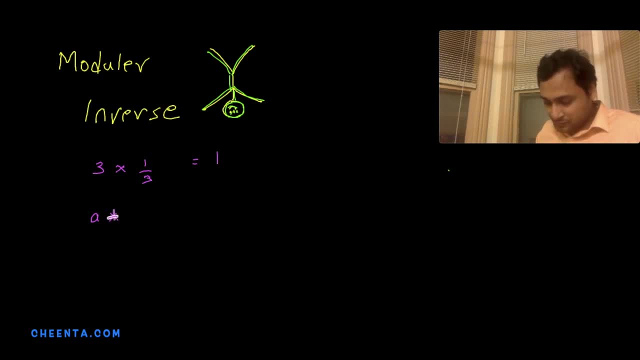 is another number. Let's call it a. to the power, a, a raised to minus 1, such that their product is 1.. We will change the game a little bit. We will restrict ourselves to only integers. So let's look at integers, But again, not all. 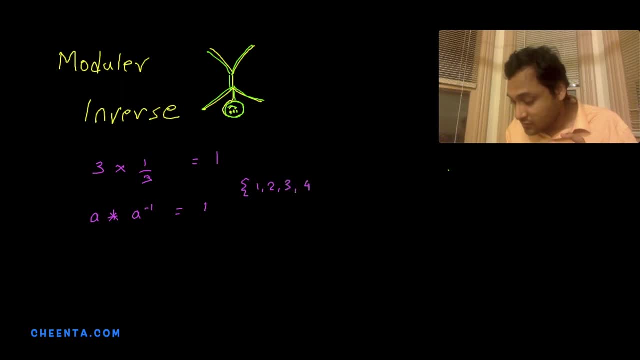 integers, Integers up to 10.. So 1,, 2,, 3,, 4,, 5,, 6,, 7,, 8,, 9,, 10.. We are not allowing fractions and we are not even allowing all integers, Just 1 through 10.. All right, We will change the. 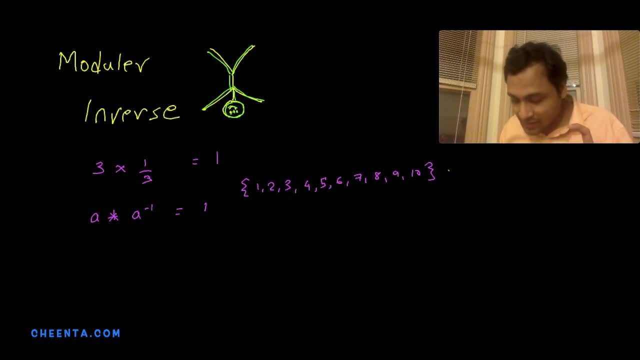 operation. So look at the example that I just mentioned at the beginning of this discussion. That's just normal multiplication. We will change the operation a little bit. So this is the new operation. The new operation is: take any two numbers, let's say a and b. 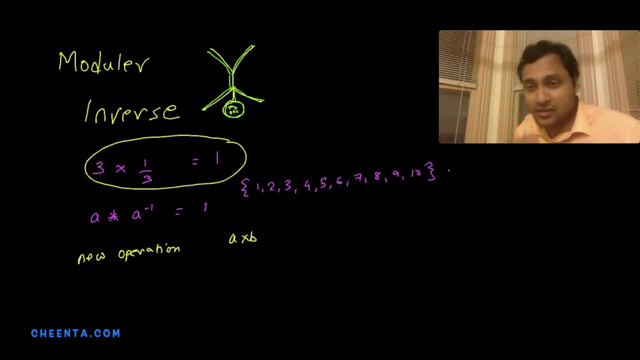 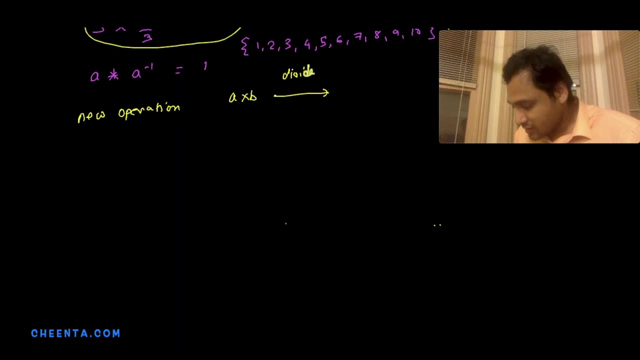 multiply them, whatever the normal multiplication is, and then divide them by 7 and divide by 10- in this case, I'm sorry, divide by 10 to compute the remainder. so that's the final output of the operation and you can try to kind of 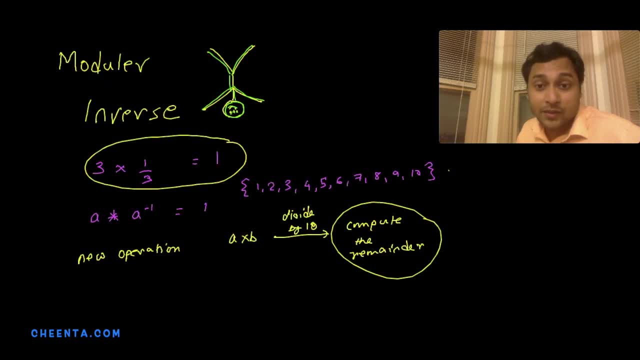 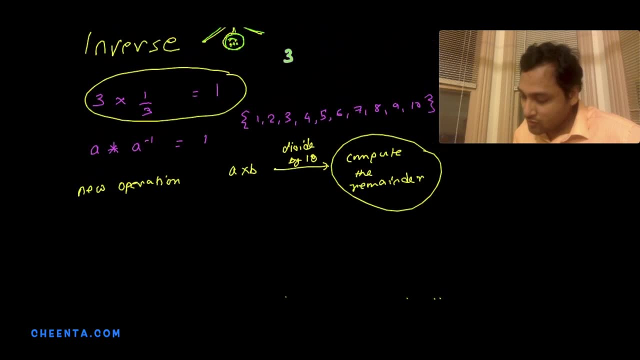 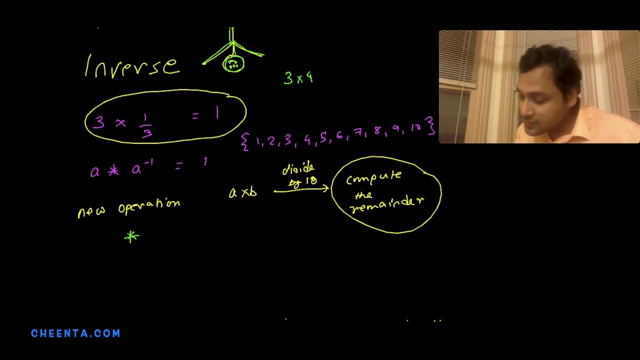 play with it a little bit, because that will give you an idea about what's going on. so let's take an example. let's take three and four. if we let's call this new operation star, so what would be three, star, four is a new operation. what would 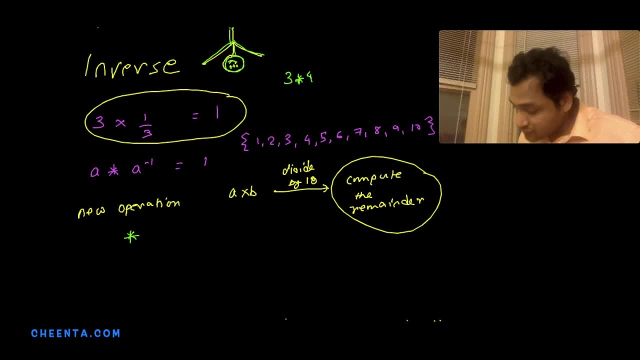 be three star four. well, three star four. you would first multiply three and four, like you do normally, so that's 12, and then you divide by 10 to compute the remainder, so that's two. if you divide 12 by two, that's 12 by 10, that's 2. so 3 star 4 is 2, that's how. 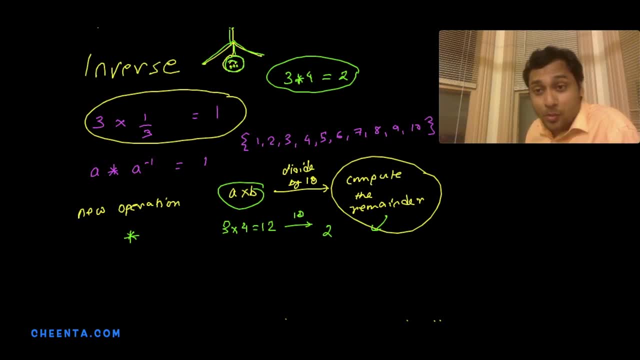 we are defining the new operation. we are not going to just do more normal multiplication. we will be doing this so-called very complicated sort of a multiplication, and this is sometimes known as modular or modular arithmetic. so if you know a little bit of number theory, you know this. ok, now the question is: is there a? 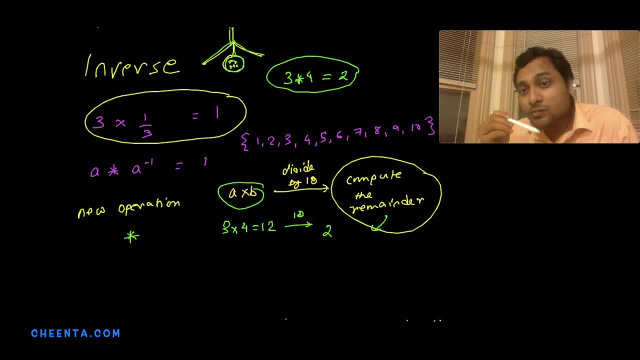 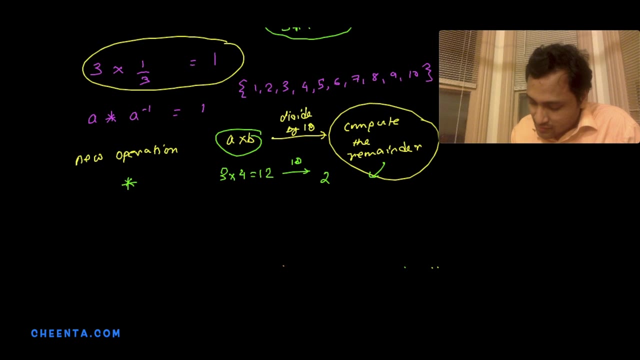 number which, when we multiply with, or do this new operation with, 3, gives a remainder 1, or the output is 1. so is there a number- let's call it the inverse of 3, whatever this net number is. in fact, I can use a fancy notation here, because 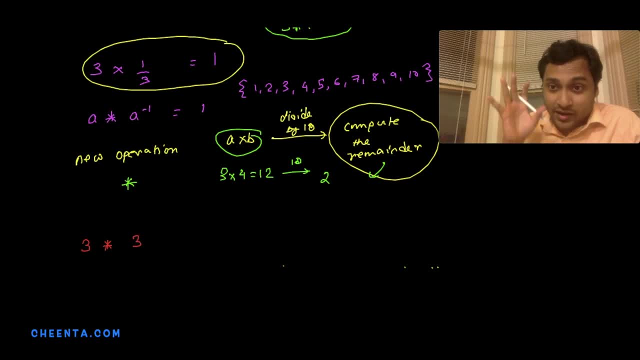 this is not 1 over 3 because, remember, we are restricting ourselves to the set of integers from 1, 1 through 10, so we cannot use fractions, so let's call it a 3 hat, so 3 star, 3 hat. can we find such a number, 3 hat, such the? oupurs of 3 is the integer of a number, so let's call it three-star, three-hat, three-star. so let's call it three-star, three-hat, three-star, three-hat. such the number, three-star, three-hat. can we find such a number? three-star, three-hat, can we? 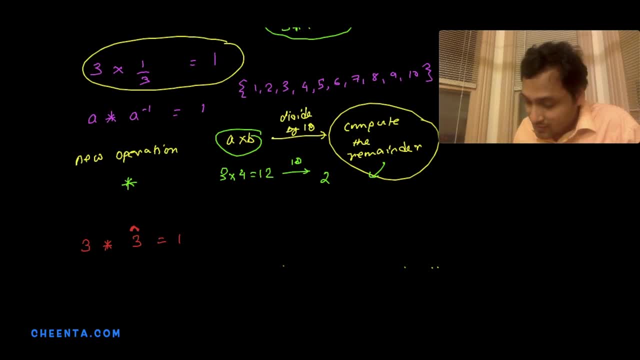 that the operations output is 1.. Is it possible to find 3 hat? Now, you can do a little bit of trick trickery here, since there are very few numbers. you can just experiment with all of them and you can actually find that 3 does have a. 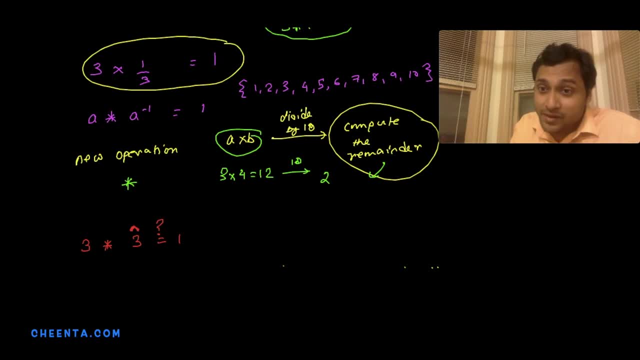 number which, when multiplied with 3, gives remainder 1 when divided by 10.. So there, 3 hat exists. Question 2, think about it again: Is there a number 4 hat, such that when we multiply 4 with 4 hat, the output is 1.. Again, multiplication.